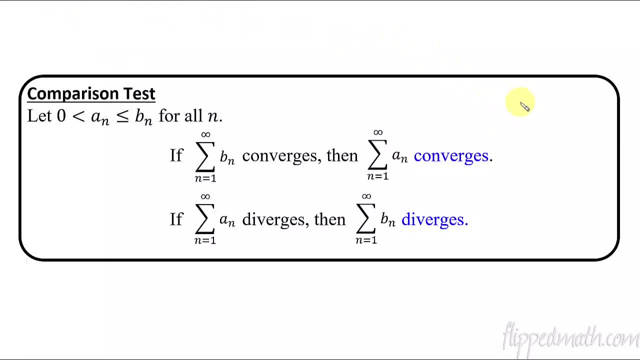 you just a little picture and I think this will make a lot more sense. Draw really quickly for this one Draw if you have some type of function that's going like this and you can see here it's going to start flattening out, kind of like this. So if you have a function that's going like this, 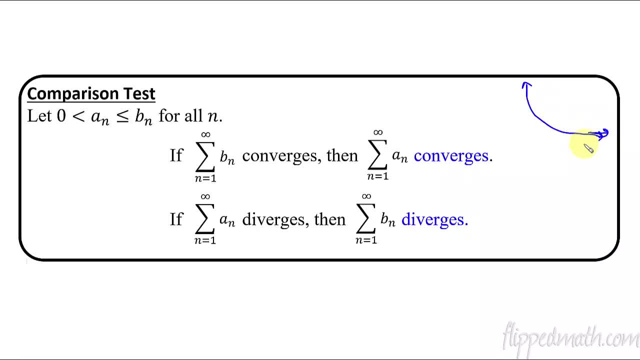 and you have a function that's going like this and you have a function that's going like this. I should have drawn it like that. It's flattening out like an exponential decay graph. This is going to converge, So we'll call this one. b of n. This is the larger one. So then underneath it, if I have, 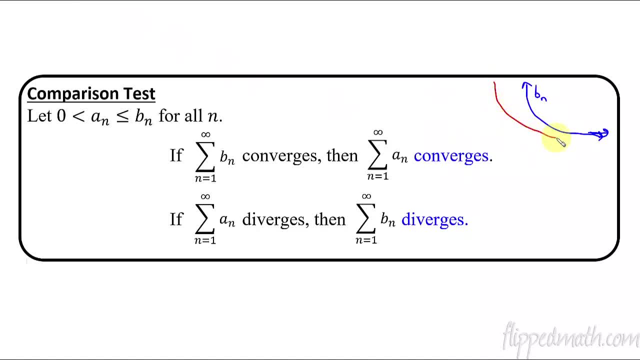 a of n and it's going like this, and then it's starting to get squeezed underneath this. this one is our a of n. Well, if a of n is smaller than b of n, it's underneath the b of n. 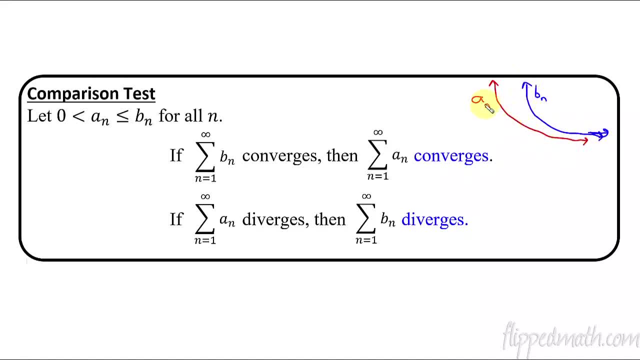 and we know b of n is converging, then a sub n also has to converge. That's what this means. If the larger one is converging, the one underneath it must also converge. So usually the picture helps you understand this a little bit more. So let's do that with the next one. If a of n is diverging. 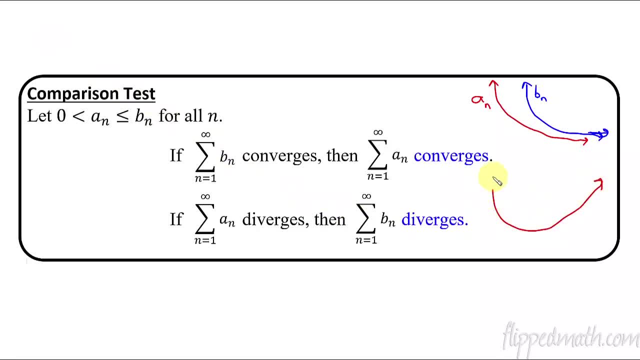 so let's say I have my a of n and it's going off forever, to infinity, something like that. So this is my a sub n, Then the one that's above it, which is b of n. if it's going like this, 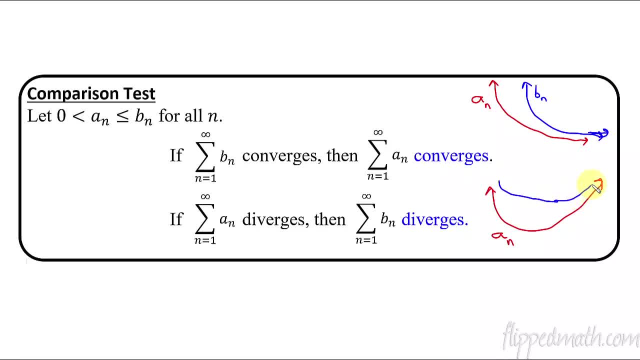 if I know it's above it, it's not going to cross it, So when it gets there it has to start going up. Then that means that b of n, so I'll call that one b. I should say b sub n. 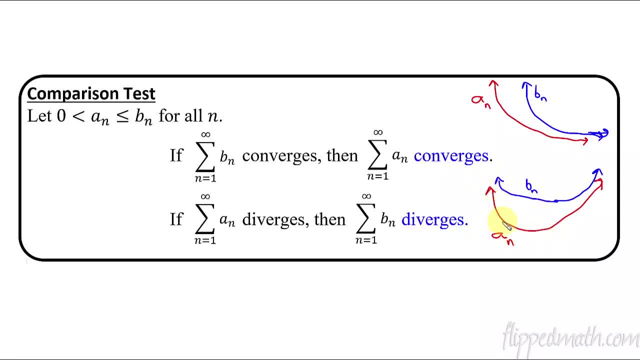 b sub n is also diverging. So if the lower one is diverging, then the one above it obviously has to stay above it, so it is also diverging. That's what this means. That's called the comparison test, And again I would think of it like graphs: The one that's above it, 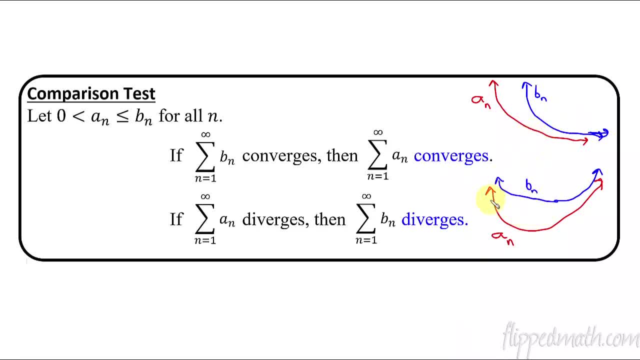 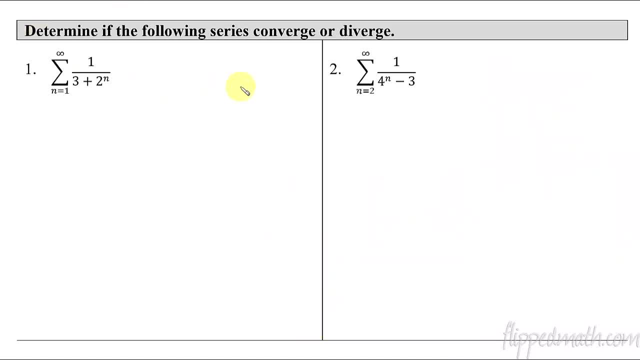 if it's converging, then the one underneath it must converge. If the one below it is diverging, the one above it must also diverge. That's what these two statements mean. All right, let's put it into practice. Let's try this out here. So what we have to do is: 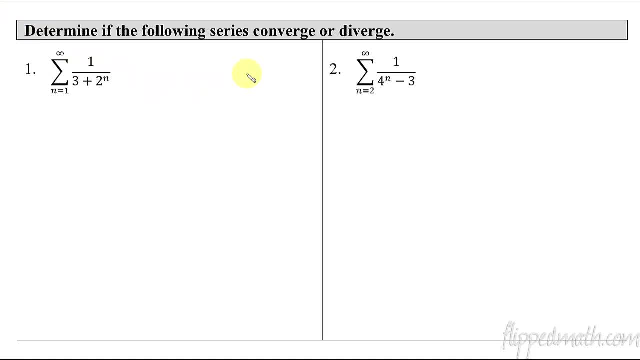 find an example of something that we can compare it to. So I'm going to take this thing and I want to compare it to. I'm going to compare 1 over 2 to the n. See, these two things look very similar. Now, which one of these is larger? I'm going to remind you of something right down here. 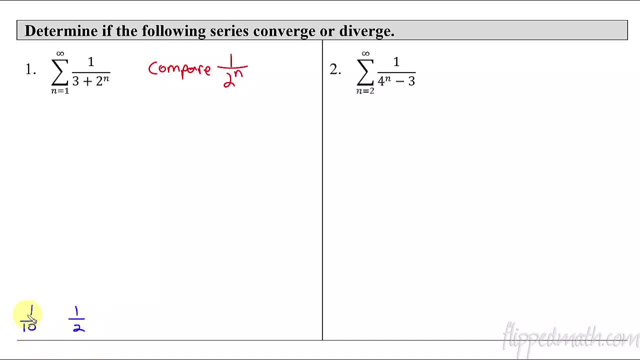 in the corner. If I have the fraction 1- 10th and the fraction 1- half, which one is larger? 1 half is larger. right Half is much larger than a 10th. So the number on bottom, if the number is: 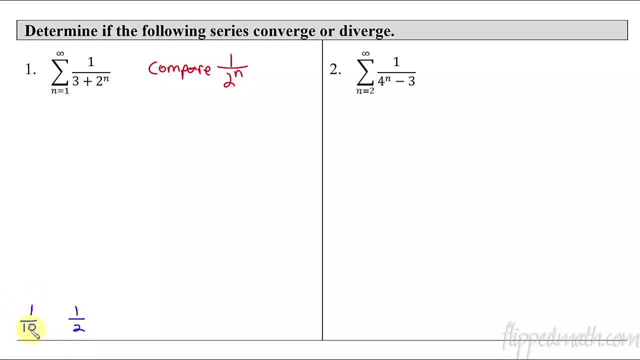 larger on bottom in the denominator, then the whole fraction is smaller. right, This is bigger than the whole fraction smaller. So look at this: This fraction has a larger denominator, which means the entire fraction is smaller. So I can say this: I can say that 0 is less than 1 over 3 plus. 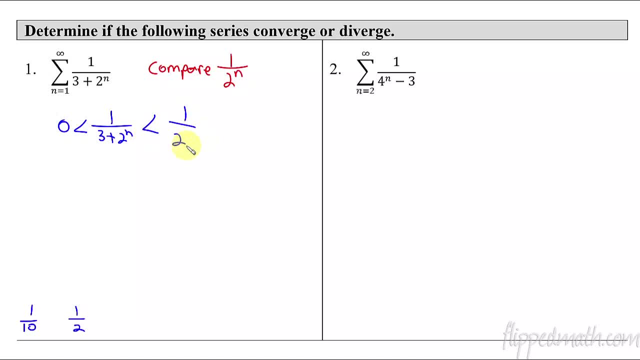 2 to the n, which is less than 1 over 2 to the n. So it goes in this order. Now, what do I know? and I know that it converges from our practice with geometric series. So that means, if this one 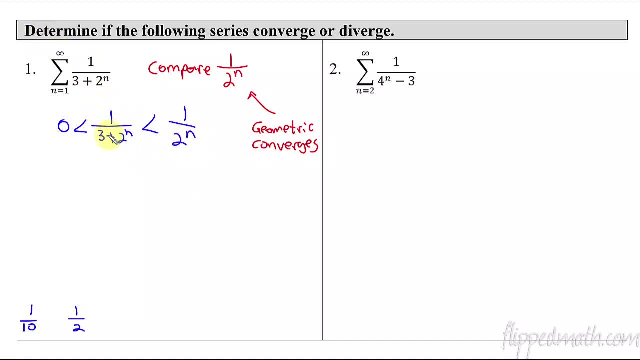 is the larger one and it's converging, then this thing must also converge, So that thing I can say converges. Why? Because comparison test. Now, if this thing that I was comparing, if this diverged, if this thing was diverging, then I could not make any conclusion about this. So you have to. 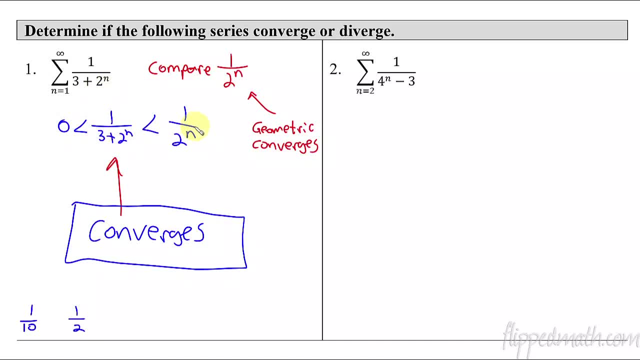 be careful about that. There would be no conclusion if this thing diverged. I would have to come up and compare it to All right, so let's do this one. So here, the most obvious, based on the first example that we did. the most obvious thing would be to compare it to 1 over 4, to the n. 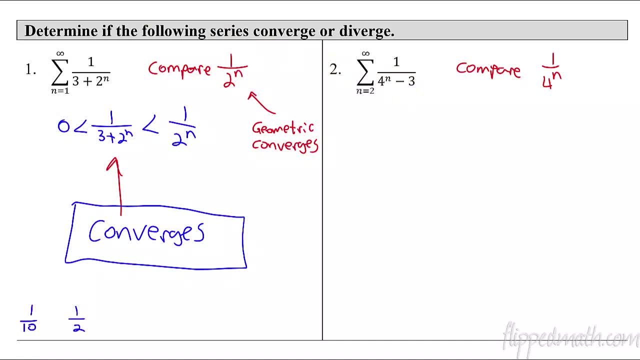 But there is a subtraction here. So when you start listing in order which one is larger and which one is not, you'd have this 1 over 4 to the n is actually smaller than this whole fraction 1 over 4 to the n minus 3,. right, Because if you're subtracting 3, that means this: 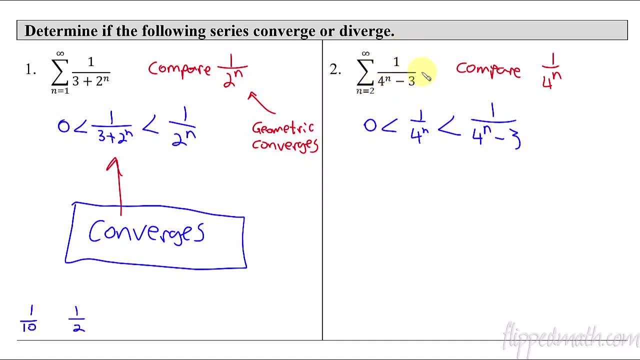 denominator is smaller than this whole fraction. So if you're subtracting 3, that means this denominator is smaller, which means the whole fraction is larger than 1 over 4 to the n. So now, even though we know this thing is, this is a geometric and it converges. So we know that. 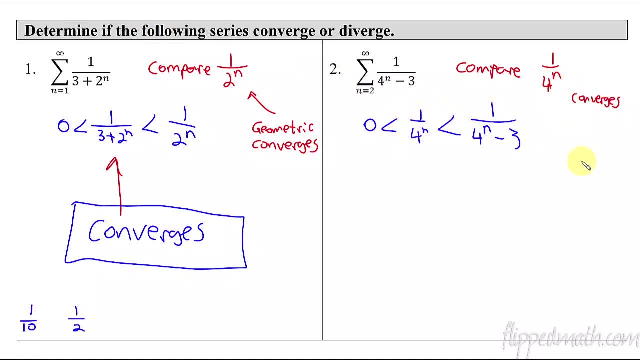 thing's geometric, it converges. So even though we know this thing converges, we can't make any conclusion about this. We don't know what's happening. The lower one converges doesn't mean the one on top has to converge. It might still diverge. So what we do is we have to come. 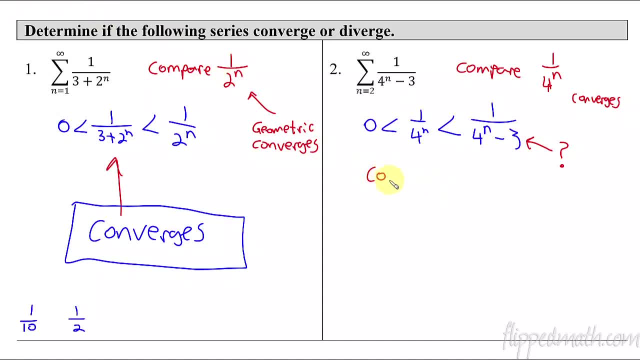 up with something else to compare it to. So let's, let's compare. Let's compare 1 over 3 to the n, Because now I can say 1 over 3 to the n is actually going to be larger than the 4 to the n, right? Because if it's a smaller denominator, then the whole. 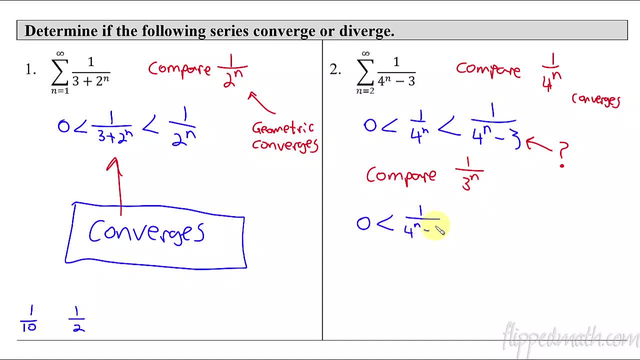 fraction is actually larger. So this now is 4 to the n minus 3, less than 1 over 3 to the n, And now I know that this converges, So this thing converges And if the one that's larger converges, 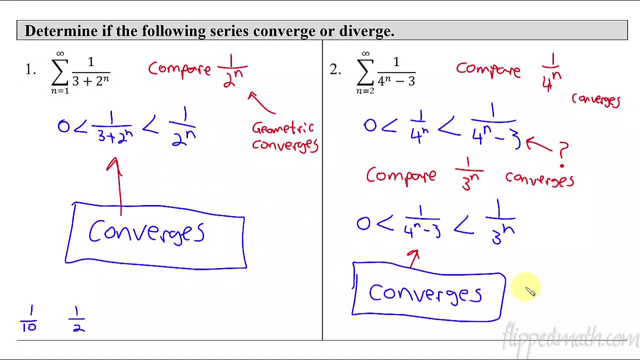 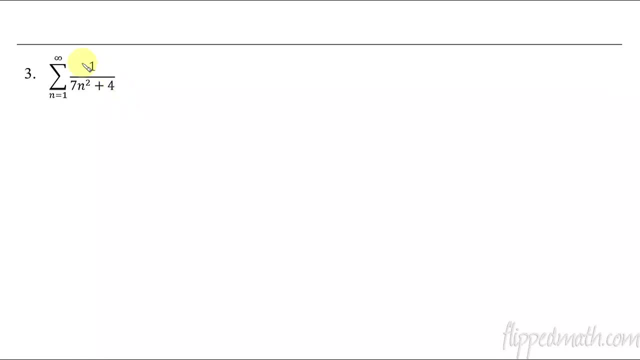 then that one must also converge. Now let's do one more example of these, And that is: you have- uh, let's see you've got one that's not exponential. so you have this thing here. let's think about what can we compare? it looks kind of similar to this. i could compare it to: 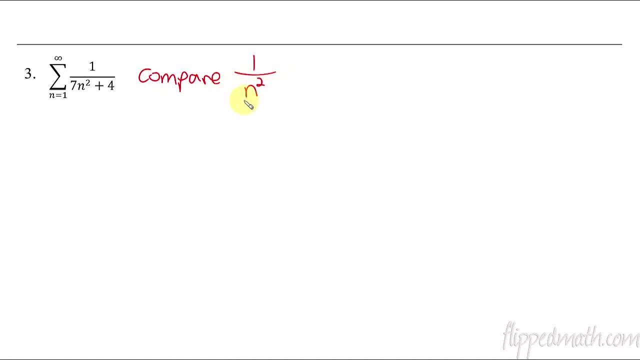 one over seven n squared. i could put the seven here, but i don't have to. i can just say n squared. i'm just trying to. the seven won't really make much difference when you're talking about going off to infinity, and this here is a p series. so this is a p series and the p is larger than one. 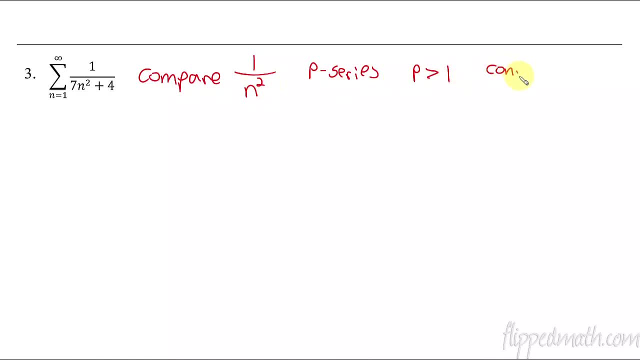 it's a two. so therefore this converges. so i know that this thing converges. so now let's compare them. so let's put them in order to make sure that we know which ones which we got more stuff going on here. in the denominator: the denominator is larger, which means the whole fraction is smaller. 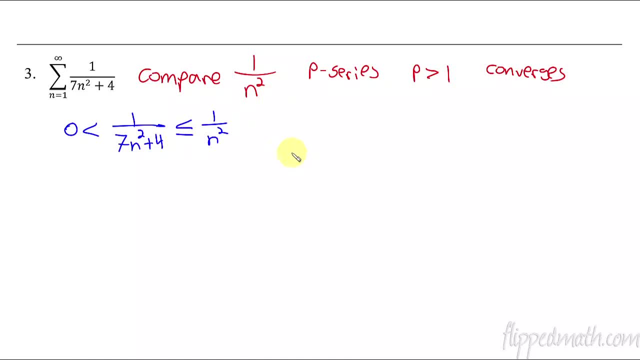 and then this wouldn't be less than or equal to the one we're comparing it to. so since this works, and we know that converges, then this one also converges. all right, so we've covered the comparison test. now, next up, we're going to take a look. 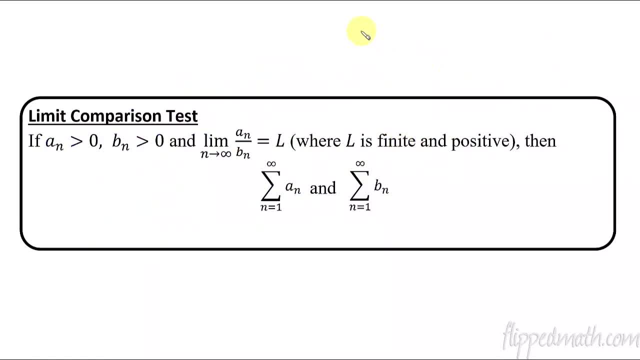 at the negative function of the differential. we're going to look at the problem as a whole. let's look at this and take a look at something in the difference between the both, and then we're going to what's called the Limit Comparison Test. I will admit, most of the problems I work through I tend to use the Limit Comparison. 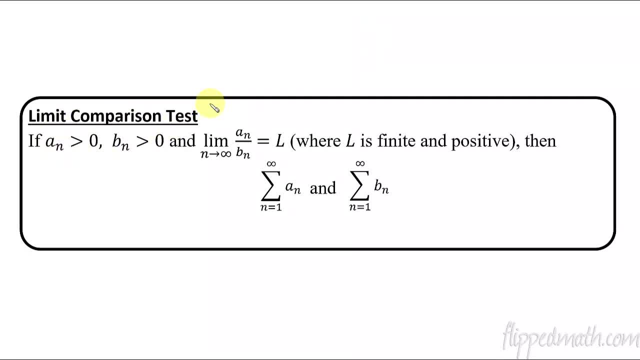 Test. I just think it's a little easier only because you don't have to figure out if A or B is larger, Which one's larger. All they have to do is both be positive and then you can work with it. See, on this other one that we worked through, we had to know that the A was smaller than 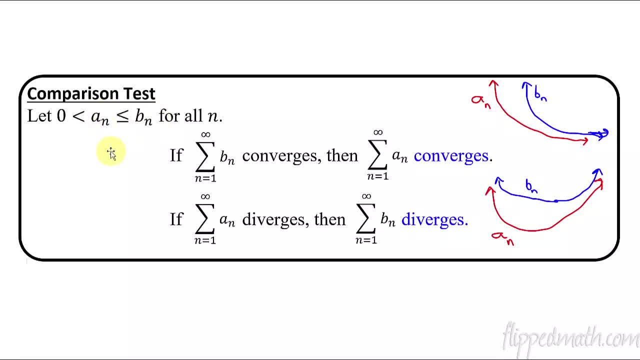 the B One of the series. we have to know which one's larger and which one's smaller to make the comparison test work. So you will have problems that you have to work with that, but I find it a little easier to usually use the Limit Comparison Test. 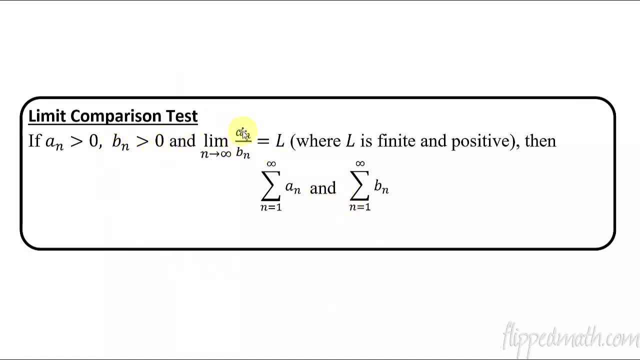 So here's what happens: You don't have to know which one's larger, You just put them in a little fraction. So you set this up, and then you take the limit as n approaches infinity, So you put one over the other, and then, as long as your limit exists, so your limit is. 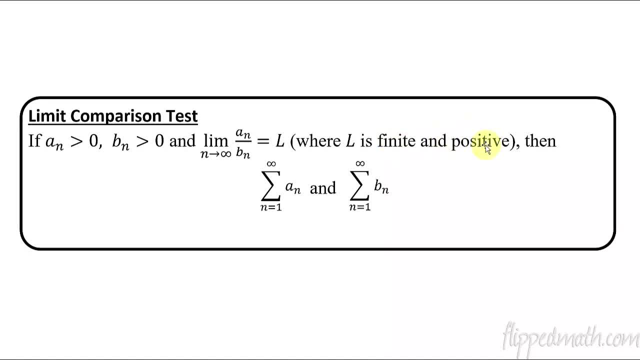 finite, it exists and it's positive. then what happens is both of these two series either both converge or they both diverge. So if you know the one you're going to compare it to, And then you take the other one, and then you take the other one, and then you take the. 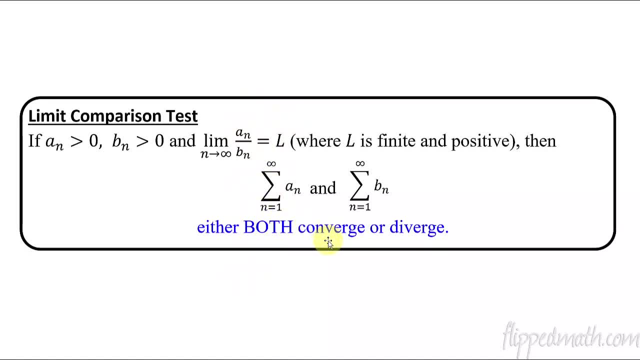 limit. If the one you're comparing it to converges, then they both converge. If the one you're comparing it to diverges, then they both diverge. So it's a bit different than the other one, where you had to know which one was smaller. 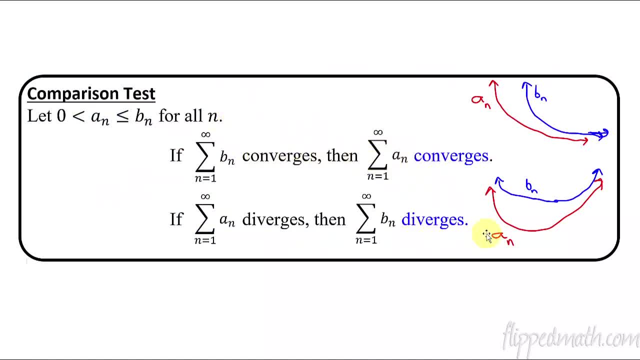 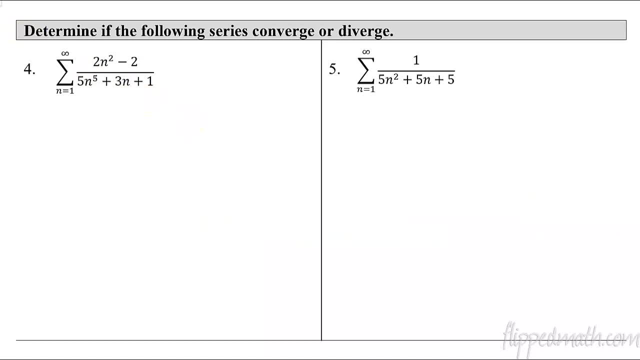 and which one's larger, And then that depended the convergence or divergence, depending on which one was on bottom or top. So this is going to be a bit different. So let's take an example with this one. So how do you know what to compare it to? 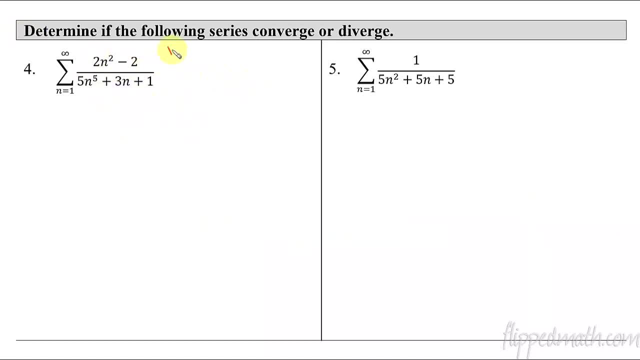 So when you have something crazy like this- here I'm going to put this in quotation marks- this idea of reducing- It's not really technically reducing, but you have to think of this like horizontal asymptotes. If you were to go off forever and ever and ever, what would you really focus in on? 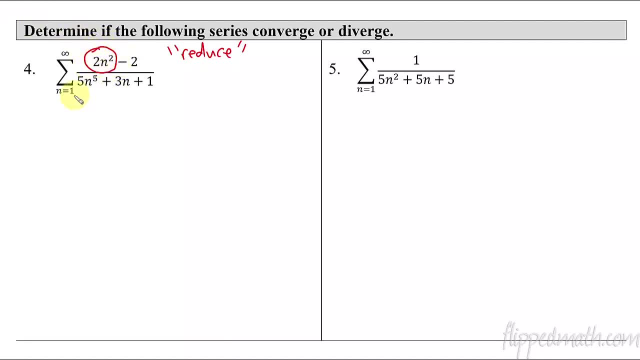 You're focused really just on the terms that are the largest terms, This term and this term. So I'm going to take this thing and just kind of reduce it down. So I'm going to compare it, compare it to. So this becomes, I could say, two over five, n cubed, like that. 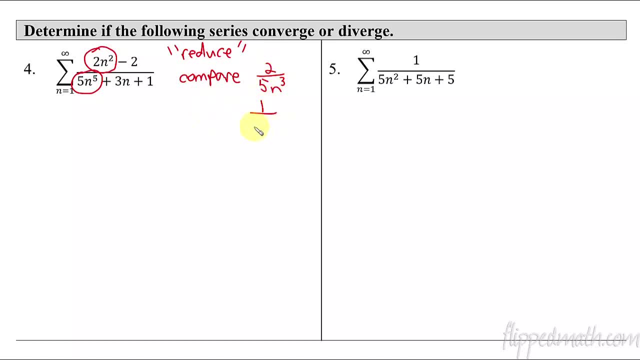 But really I don't even need the two fifths. So I'm going to take this thing and just kind of reduce it down. I could just say one over n cubed. I don't even need the numbers there. So this is what I mean by quotation marks: reduce air quotes. I'm doing, but you can't. 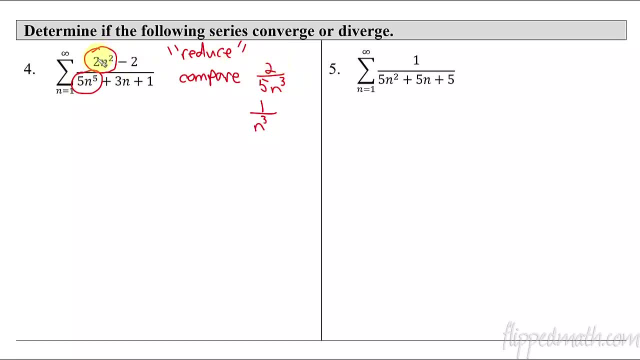 see me, And that is that you just reduce the largest terms to kind of figure out what you can compare it to. So now we have this thing, this one over n to the third. You could also do two fifths, two over five, n to the third, but it's not necessary. 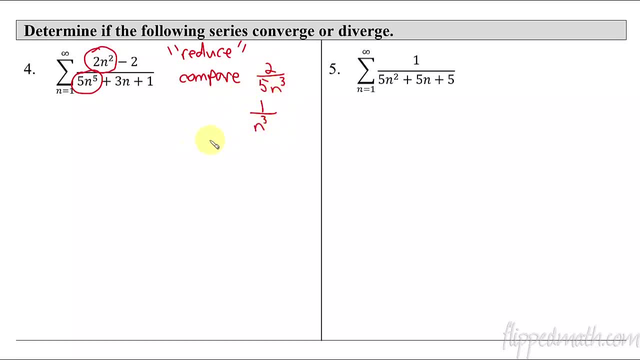 You can just do this one. So now, does this converge or diverge? This is a P series and it converges. Okay, So we know that this thing converges, So now let's set up our limit. So we're going to say the limit is n approaches infinity. 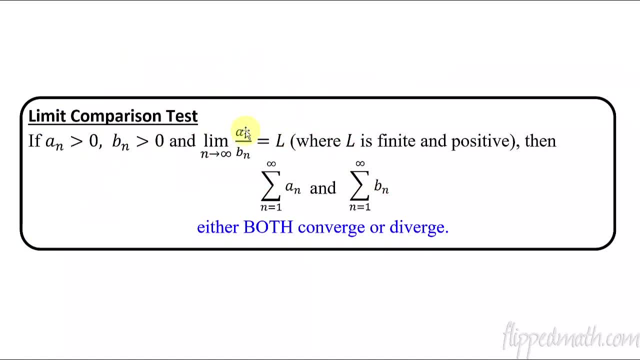 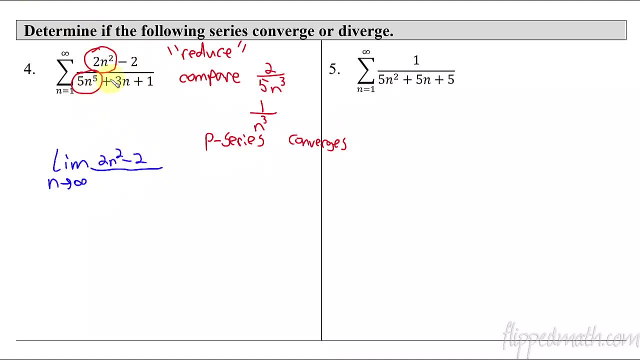 And what we do. if you look back, here we're going to set up one of them over the other, So I just start with the one. that was the one that they gave us. So the limit of two n squared minus two: all over this thing, five n to the fifth plus. 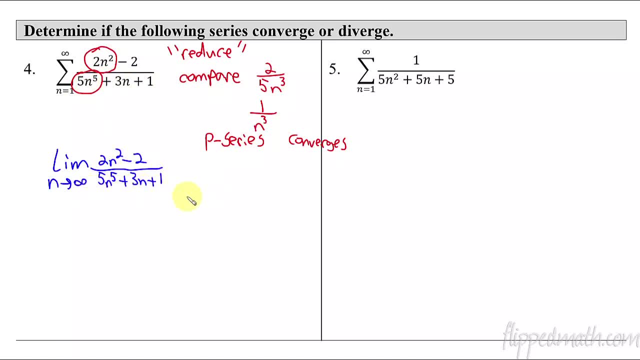 three, n plus one, And now we're going to divide it by the one we're comparing it to, which was this one right here. So we're, instead of dividing, though, let's just multiply by the reciprocal, because that's much easier than dividing fractions. 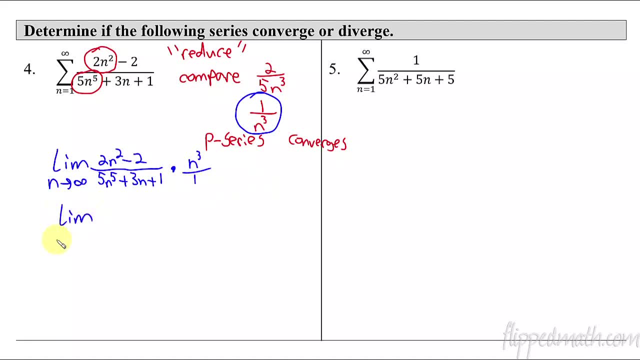 Multiply by the reciprocal, So that now gives us the limit as n approaches infinity, of the n cubed distributes. That gives us this new fraction And then that whole thing equals. remember your horizontal asymptotes. you're only worried about the end of the fifth. 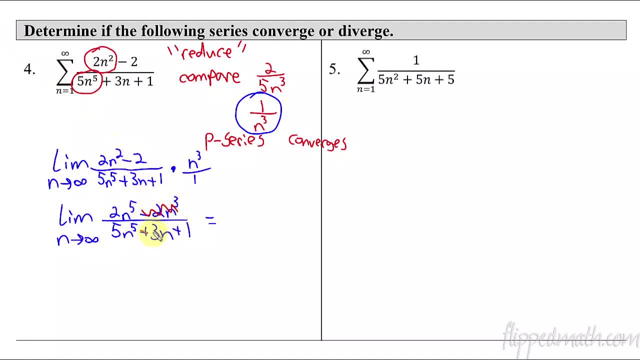 None of this stuff matters, right? You're going off to infinity. So blah, blah, blah, blah, blah blah. We don't care about it. So it's just two fifths. Now, it's not necessarily that we care that the answer is two fifths. 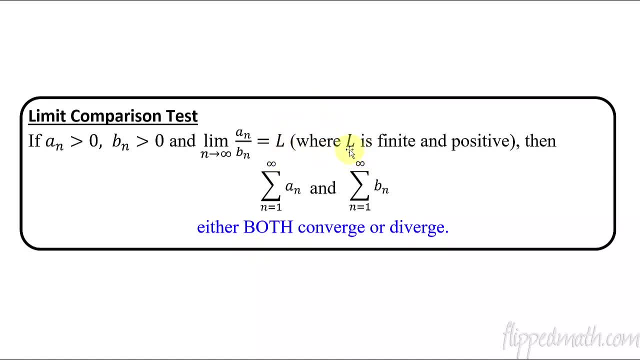 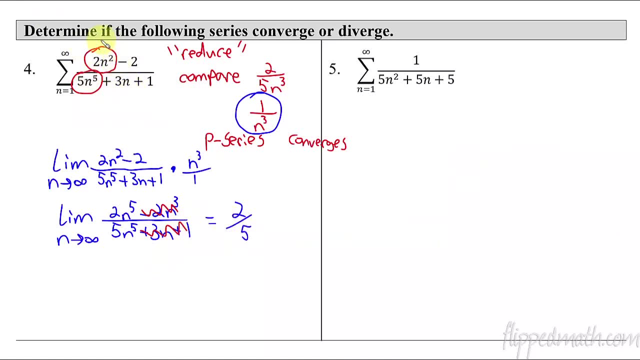 It's just that we care that the limit existed, that the limit is finite and it's positive. And so, since it works, Since it is finite and it's positive, then what we know is that this convergence is the same as this convergence. 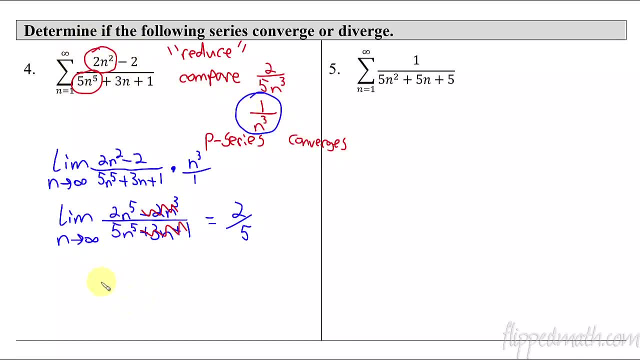 So since this one converged, they both must converge. So our answer is that our original series converges. Sometimes in my answer key I might've put both converges, but it's the same thing, You know. we're just saying: if they both converge, then this one is obviously converging as well. 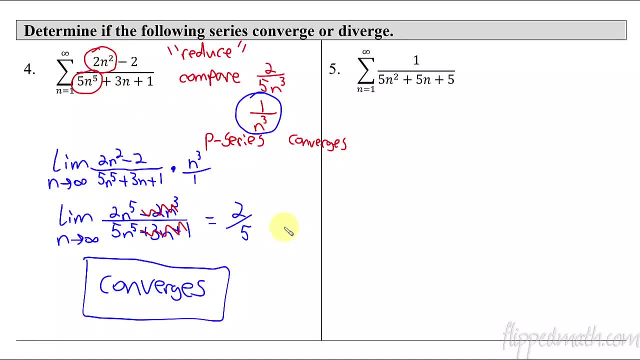 Okay, So that is how the limit comparison test is. Don't be confused with the comparison test which we did the first one. So let's look at this one now. So we're going to use some type of reduced comparison, So let's compare what's something that would be reduced from this. 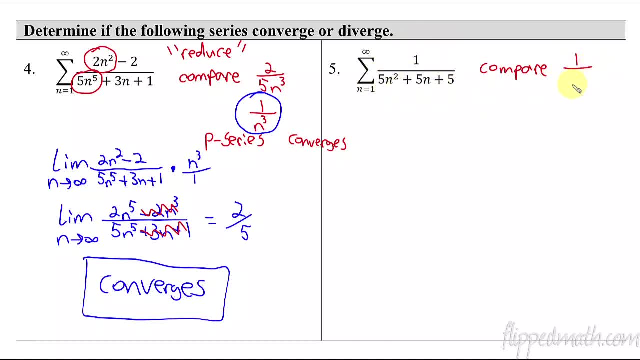 Well, we just are going to look at this largest term, and I can get rid of the five there. Let's just do one over N squared. That's all we need to use to compare. Now is this. before we start working it, we need to know if this converges or diverges. 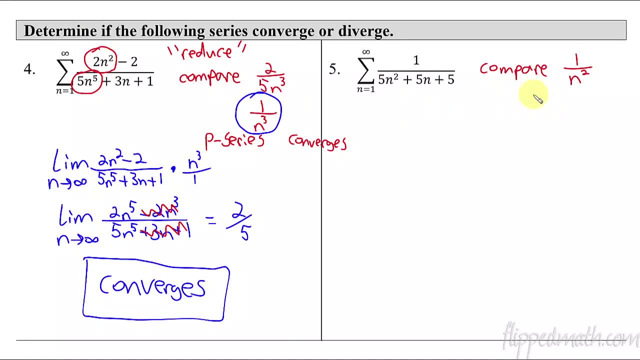 This is a P series. I don't know how to I actually started spelling P, sorry, P series, and the P is greater than one, So that, therefore, this thing converges. So what's nice about these tests is you get really good at the stuff we've already been. 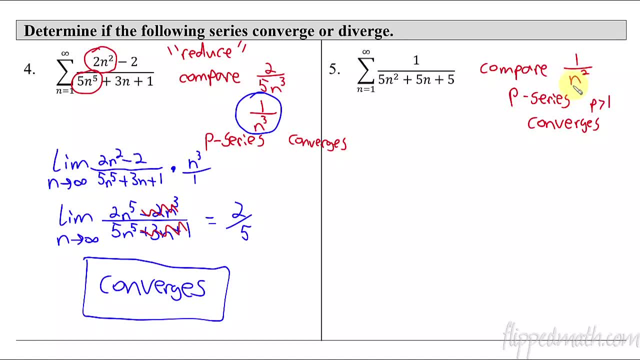 practicing in unit 10, the geometric series, the P series, the term test. you got to know all that stuff to be able to do these correctly. So you get pretty good at it through this lesson. So now let's set up our limit. 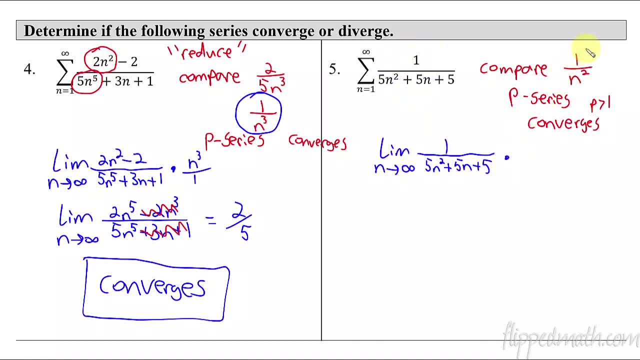 So let's just rewrite this whole thing, and then we're going to multiply it by the reciprocal of the one we're comparing it to. So there we go, And now you can see here. what is this limit going to equal? Well, we're going to have the N squared on top of five N squared on bottom. 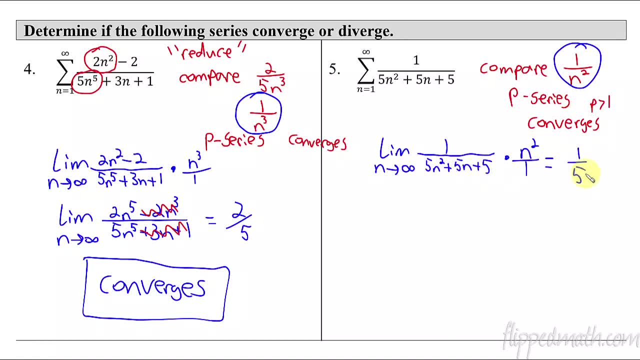 None of this stuff matters, because we're going to infinity. So it's just one fifth. So one fifth is positive. The limit exists. So therefore they both do the same thing, which was converges. So these? the answer to this is: this series converges because we did the limit comparison. 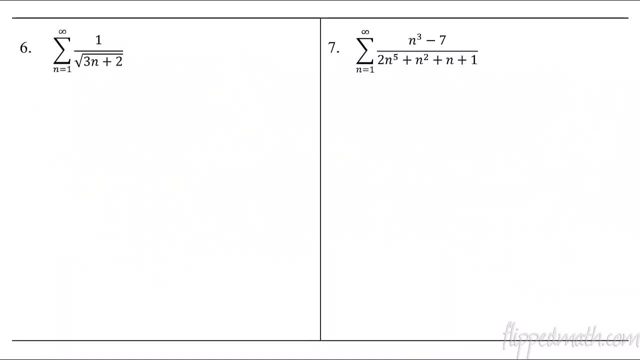 test. All right, Another one. So for this one, what do we want to compare? So you look at the largest term, which is, in this case, is this square root of three N, the. whenever we have the coefficients, they really don't matter, for when we're comparing. 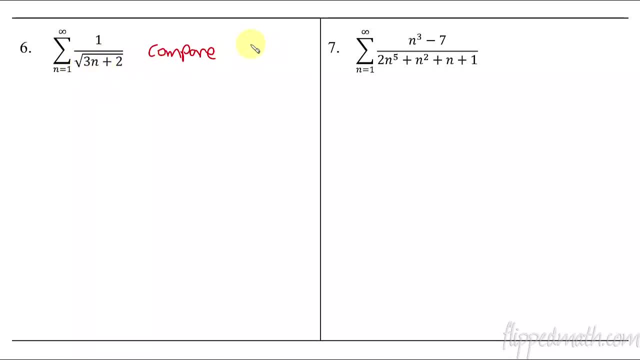 So I can just get rid of that. So I'm going to compare it to this. would be like my quote: unquote reduced: Okay, The square root of N now does this thing- I'm going to compare it to this- but does this. 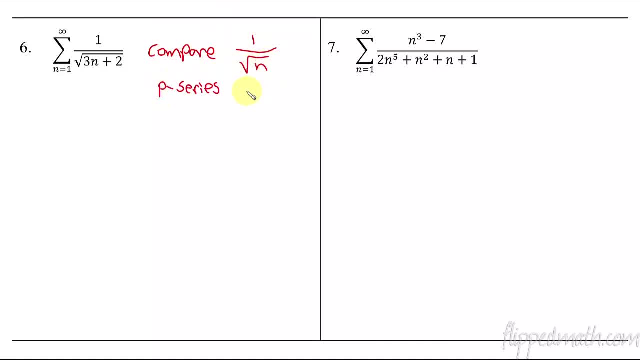 thing diverge or converge. This is also a P series, but in this case the P. this is N raised to the one half, So it's in between. it's less than one, So it's in between zero and one. So therefore this is diverging. 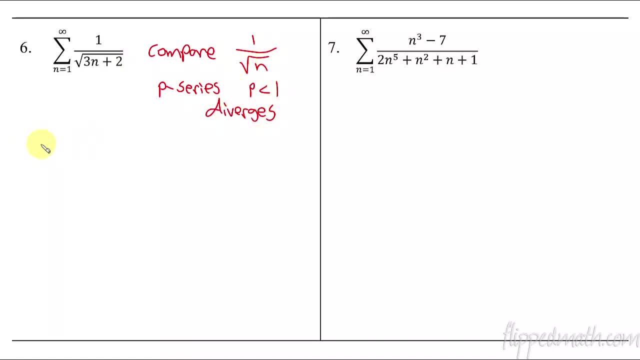 So it diverges. So when we do our limit now, if we get our limit, then we know that this thing also diverges. but let's find out first. So our limit, and it's going to approach infinity of this thing multiplied by the reciprocal. 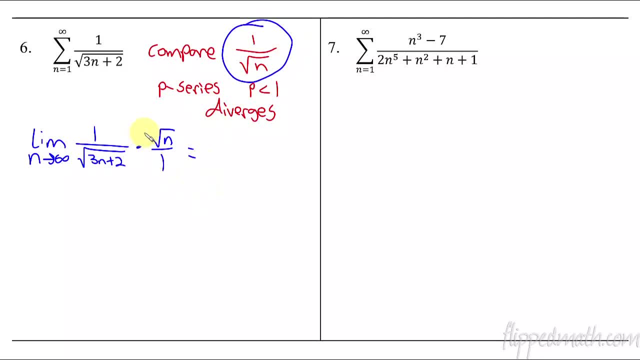 of the one that we're comparing It too, And then so you're going to get, as you go to infinity. you have to think: what is this? that we have the leading coefficients, since the degrees are the same. this is just going. 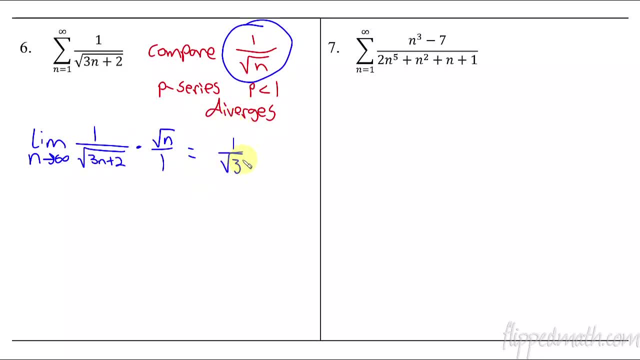 to be one over square root of three. All right, So since that's finite and positive, then the answer is that they both diverge. So this series diverges, All right, This one, let's compare. let's see, we have this term and this term. those are leading. 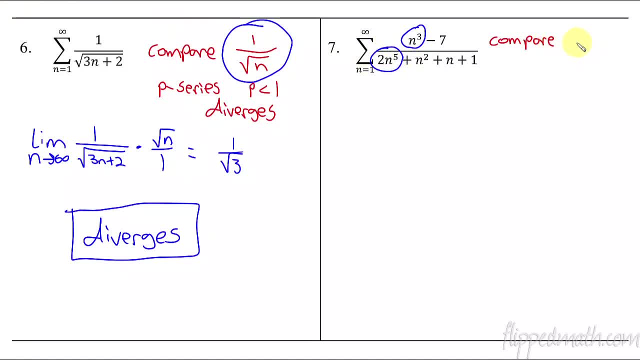 terms. So if we try to reduce those then we can compare it to one, One over. and the numbers, the coefficients, we don't care about those. So we just think about one over N squared. This is a P series that not diverges, it converges, because the P series you have P that is larger. 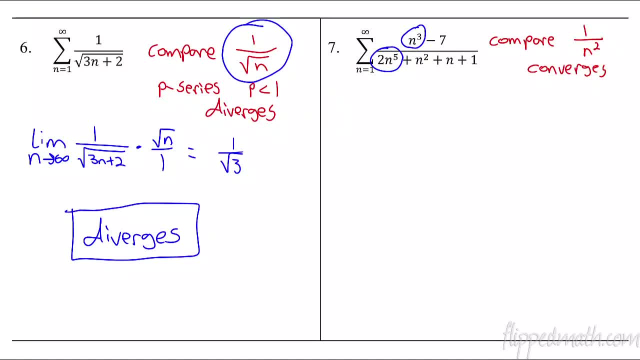 than one the exponent there. So let's check with the limit now. So we take the limit as N approaches infinity of this whole thing, and then we multiply it by the reciprocal of the one we're comparing it to, So N squared over one, and then you can see here that this simplifies down. 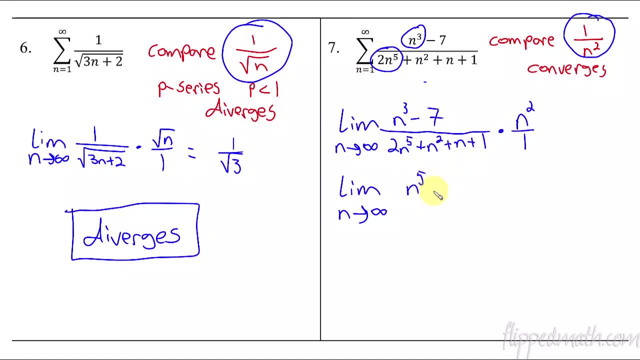 Now Let's say that it's N to the fifth minus blah, blah, blah, because the other step doesn't matter. all over, And then on bottom I have two N to the fifth plus blah, blah, blah. none of that stuff. 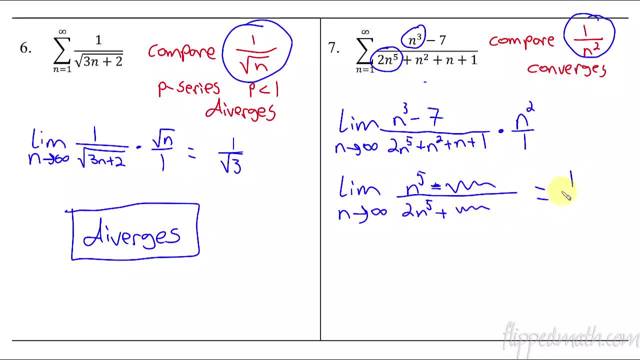 matters, because I'm just going to infinity. So then this equals one half. Okay, So we have one half, which means, since it's it is the limit, that's positive. therefore, they both are doing the same thing, So it converges. 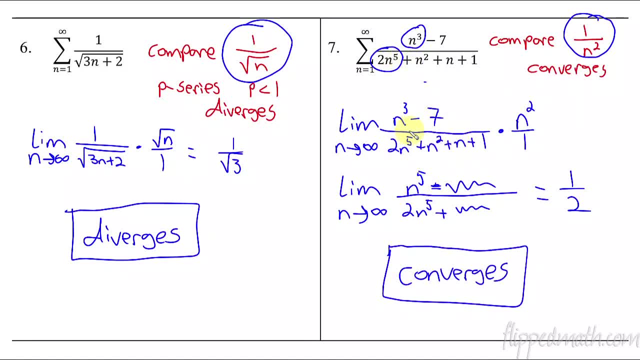 See, I like the limit comparison test because it's kind of nice. You don't have to figure out which one's larger or not. Okay, So just two more examples. I'm doing so many because there's just so many different types. 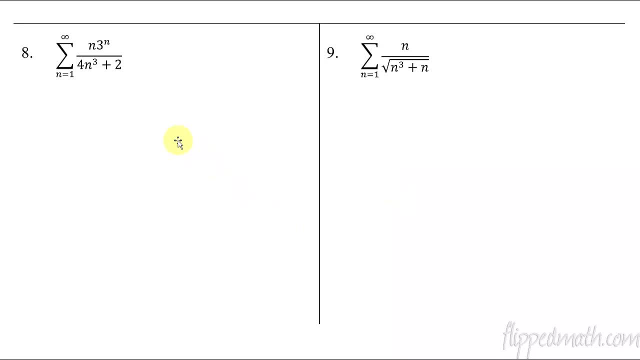 You might be faced with, and I wanted to give you a good feel for what you're going to be faced with. All right, So this one. now we have something crazy going on. So we have this term here. this is one term and we're comparing it with this term. 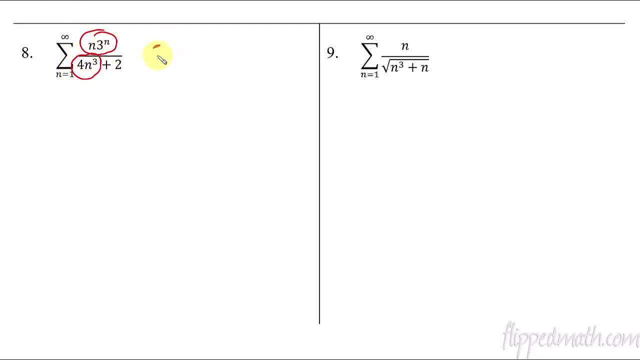 So when we quote, unquote, try to reduce this, what are we comparing? So one of those ends would cancel and we're left with three race of the N over. And now again, I don't have to do a coefficient, I can just leave the four off and just say N squared because that one of those ends canceled. 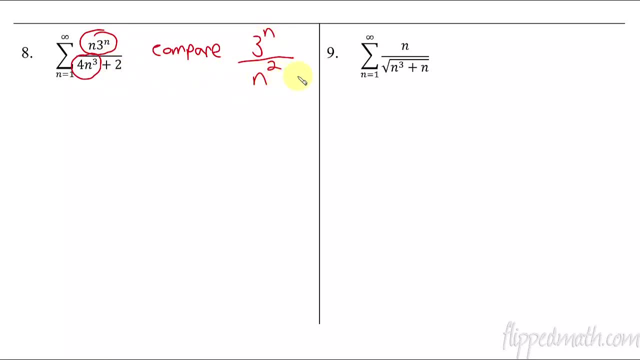 So this is what I'm comparing it to. Now, what does this do? Does this converge? Does it diverge? Because we have to figure that out before we start working through, because if we do the limit and we find out that we find the limit, but that doesn't tell us anything unless. 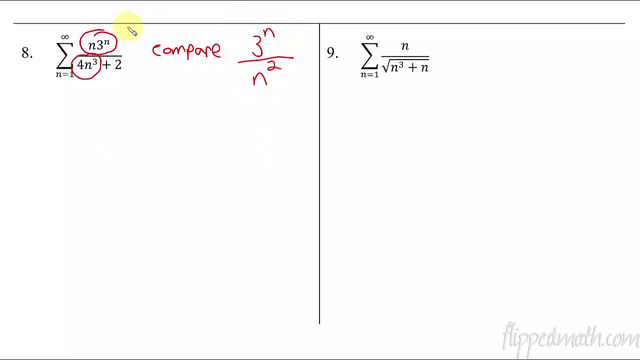 we know what this does, So this one's a little bit trickier. but if you remember the Nth term test, do you remember that The Nth term test, If you take the limit of this as N, approaches infinity. so I'm going to do the limit of. 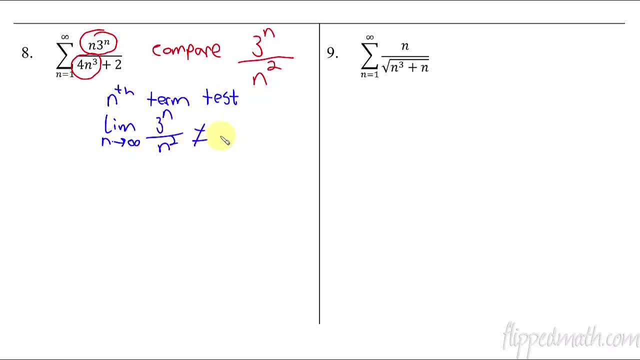 the whole thing and that does not equal zero. Now, when the limit does not equal zero, it guarantees to diverge. If it equaled zero, that doesn't mean it converges. That's the Nth term test. The Nth term test. we're just going to go off to infinity. 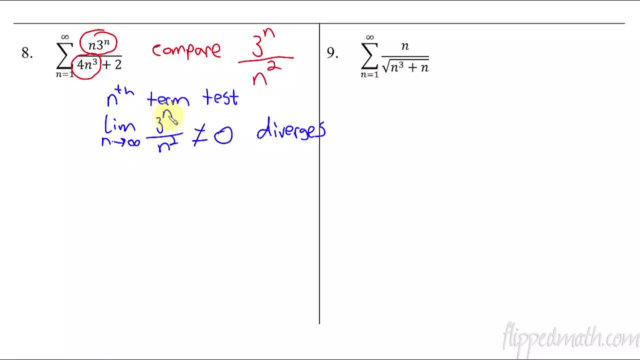 If it doesn't equal zero, which in this case it wouldn't- this thing's growing faster than the one on bottom. So then, therefore, we know for sure it diverges. So now we can use the limit comparison and set up the original one. this whole thing. 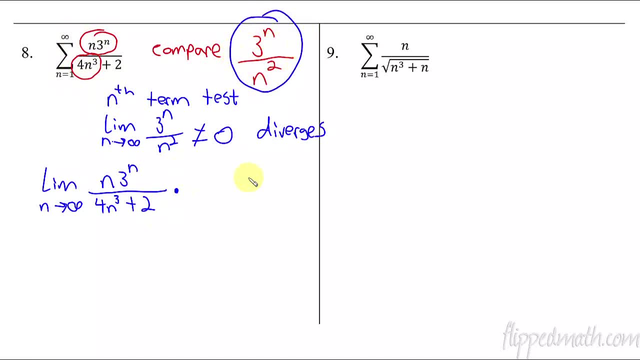 and multiply it by the reciprocal of the one we're comparing. So in this case it'd be N squared over three to the N. So now I have the limit. N approaches infinity. and then I can see here that that three to the N and that three to the N are going to cancel, and I end up with an N cubed on top. 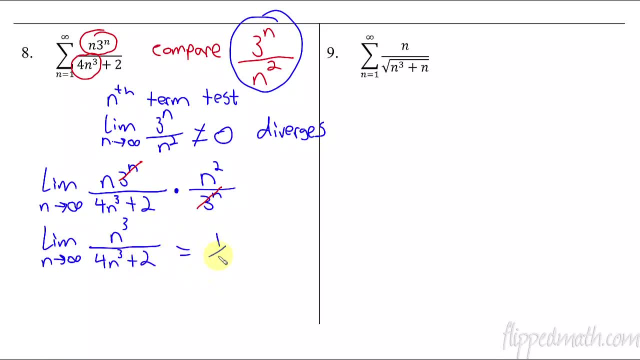 four N cubed plus two on bottom, and that will equal one fourth. So I have a finite answer. It is positive. Therefore, these are both going to do the same thing. Both are going to diverge, So this series diverges. 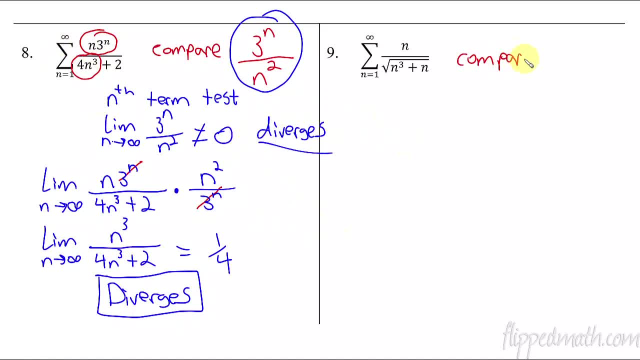 Whew, All right. Last one, Let's compare this one to okay. so I'm going to look at this N and this. Here's what I'm thinking. I'm going to take N to the first power and subtract the exponent of this. 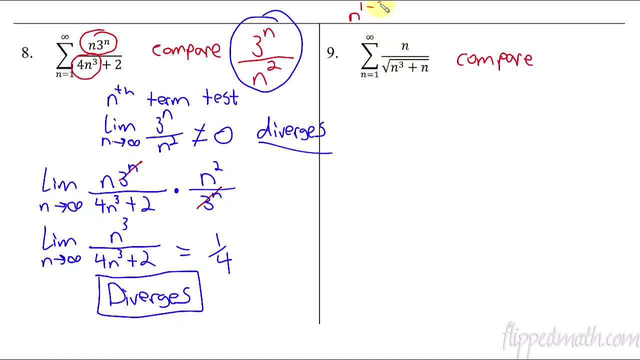 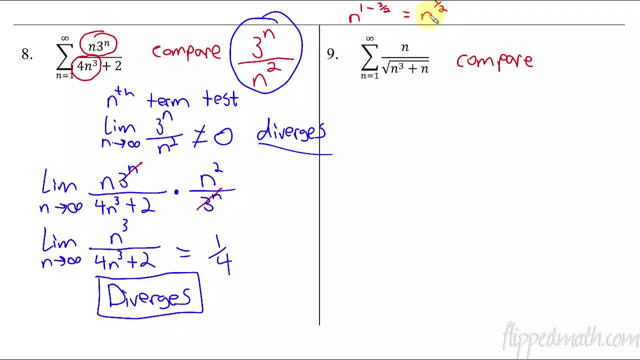 So that is three. It's a square root, So it's three halves. So one minus three halves equals N to the one half. Negative one half. Yeah, Negative one half, All right, So I'm going to compare it to one over N to the one half. 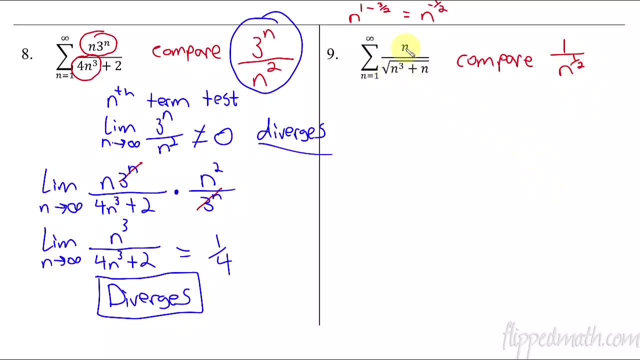 That's what I'm comparing it to. Okay, So it's like I simplified the terms that are the largest terms. Okay, So now this is a P series. Okay, So this one diverges or converges. This is a P series where the P is less than one. 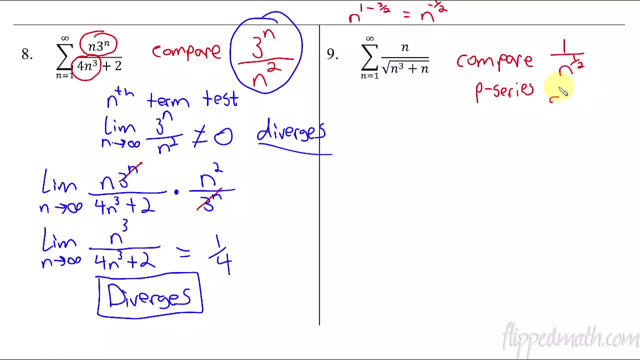 It's in between zero and one, So this is going to diverge. So now let's figure out if this one also diverges. They both diverge if the limit is finite and positive, So we'll take the limit. N is going to approach infinity of this original. 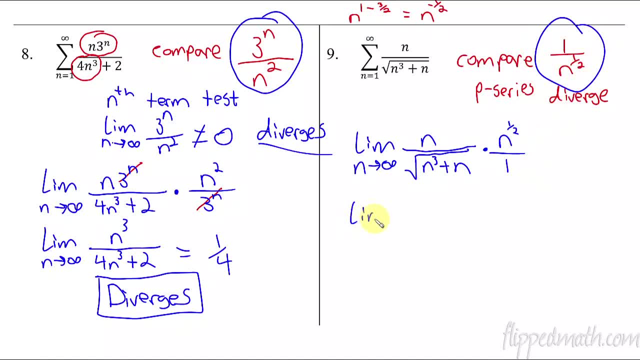 We then multiply it by the reciprocal here, Then this cleans up to be and approaches infinity of. So this is now N to the three halves on top here And on bottom The square root of N, cubed plus N. Well, now this part of it doesn't really matter, right.